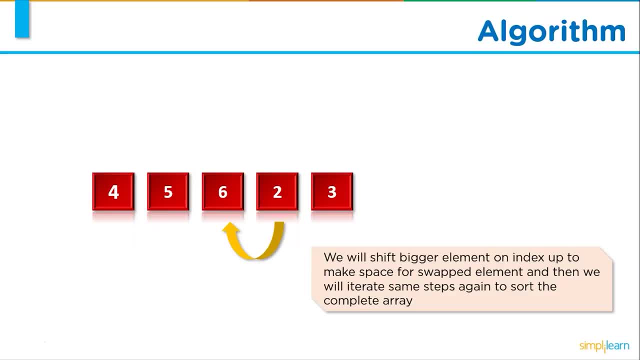 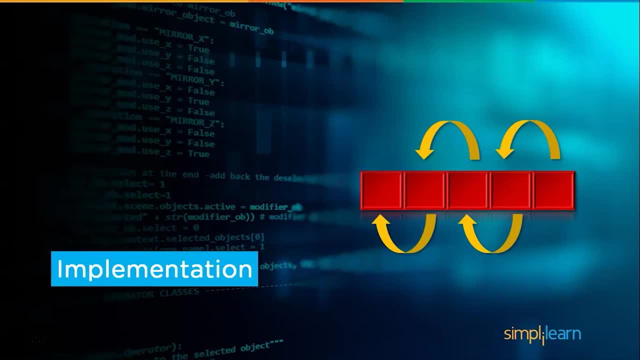 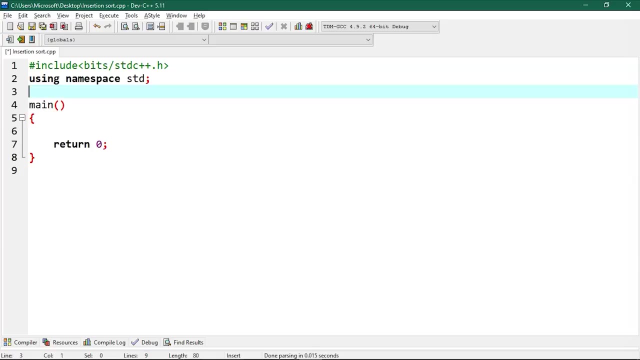 element, and then we will iterate the same steps again to sort the complete array. We have now introduced the Insertion Sort and its algorithm. Now let's implement this algorithm. We will start with creating a function to sort an array using Insertion Sort. 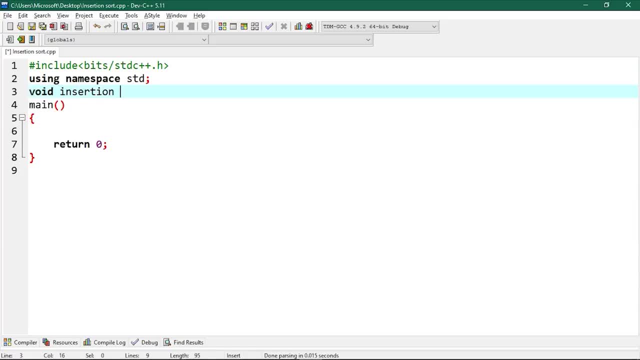 So void InsertionSort. we will give it argument as int- ArrayArr int size. We will give it argument as int ArrayArr int size. We will give it argument as int ArrayArr int size. We will declare variables: int i key j. 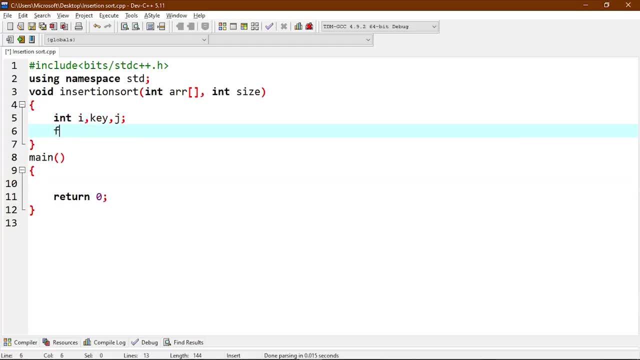 Now we will create a loop for loop from i is equals to 1 to i less than size i++. Here we are traversing this array. So what we will do is as follows: and start: relieve the ArrayArr problem with previous components. Now we will remove the parallel functions. i key j height from index 1 to the size. 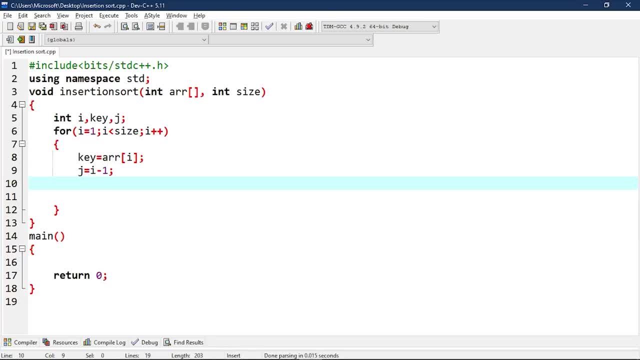 n-1.. So the key is equals to arr at. i So v is equals to i-1.. So v is equals to ae attack. i So v is equals to. j is equal to ae frame, So v is equals to ae plus. at the vector z, which is i-1, and j is equals to ae minus. 1. So v is equals to ae, x toatively raised to i-1, and j, is is equals to i-1.. So we will now remove the variables int Arrayiegmr to such that the keyword is always put it together in the array and komma duck bya bya as lines E. 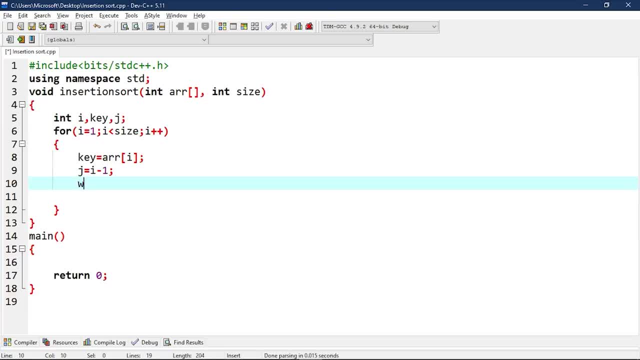 to one position ahead of the current position. so while J is greater than equals to zero and ARR at J is greater than key, then we will swap these. so ARR at J plus 1 is equals to ARR at J and J will be equals to J minus 1. 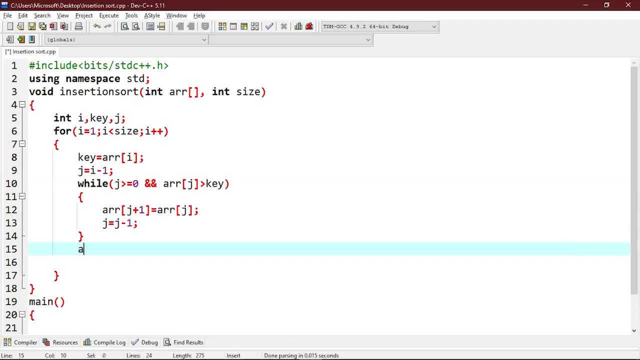 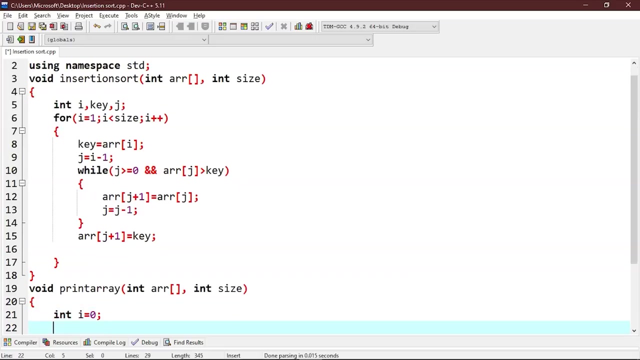 and then we will assign ARR. J plus 1 is equals to key. now we will write a function to print this array of size void print array. we will give its argument as int array and size size we will declare int i is equals to zero and for loop. 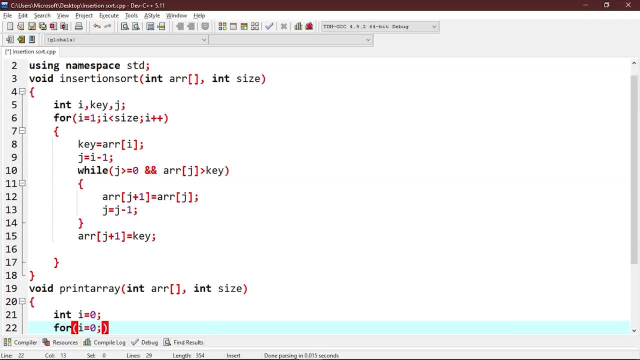 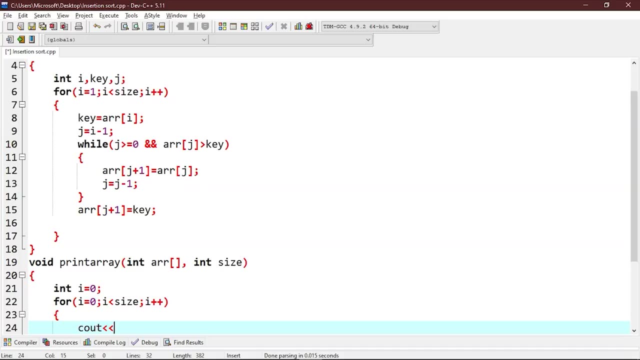 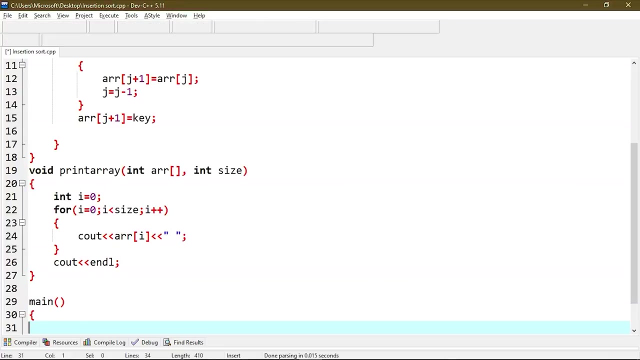 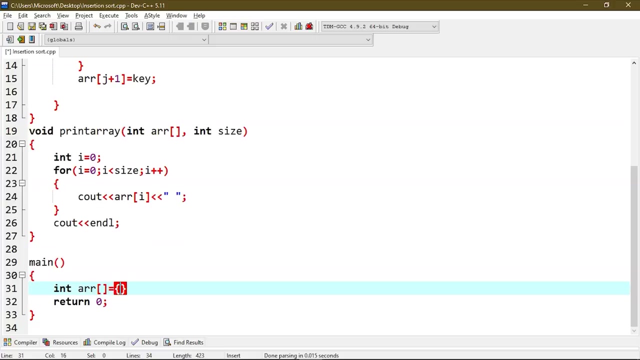 i is equals to 0, i less than size i plus plus C out ARR, ARR. Now we will write the main block. So int arr is equals to 12 comma, 11 comma, 15 comma, 9 comma, 6 comma, 7.. And size is equals to. we will find the size using sizeof. 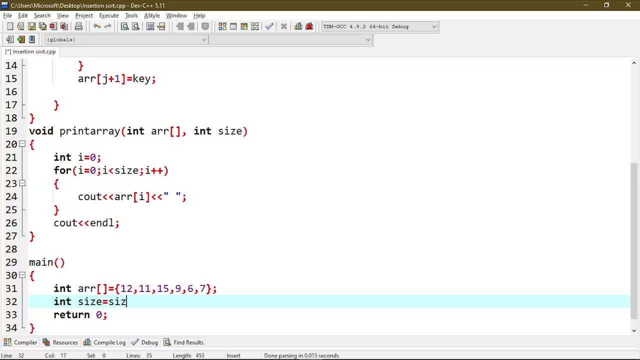 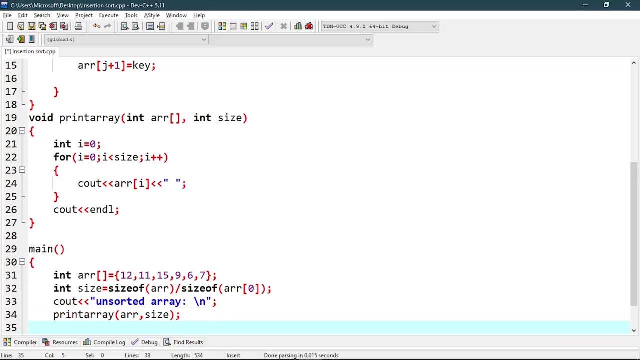 So size is equals to size of arr divided by size of arr at index 0.. Now we will print this array without sorting. See how We will print this array without sorting Unsorted array And we will print array error: comma size. 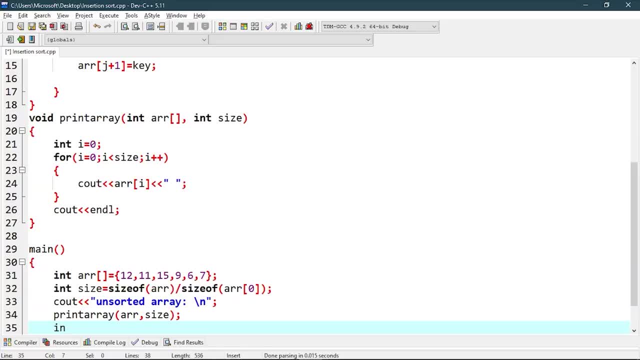 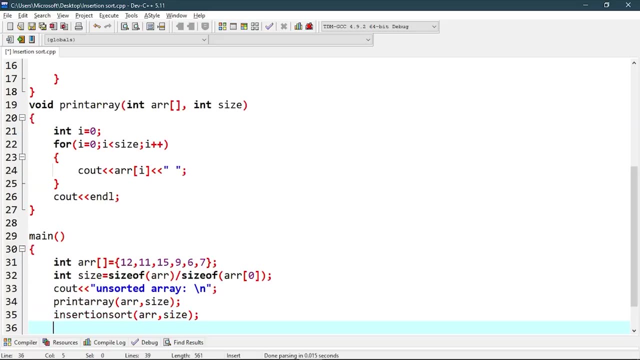 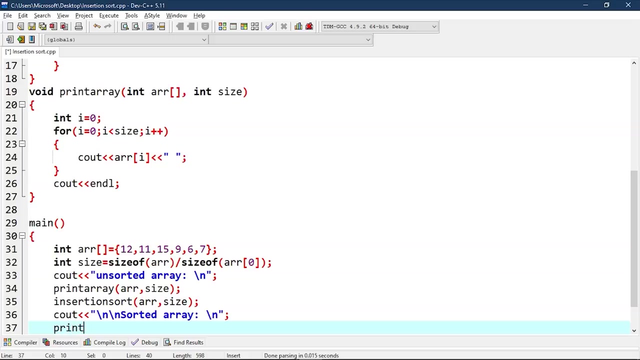 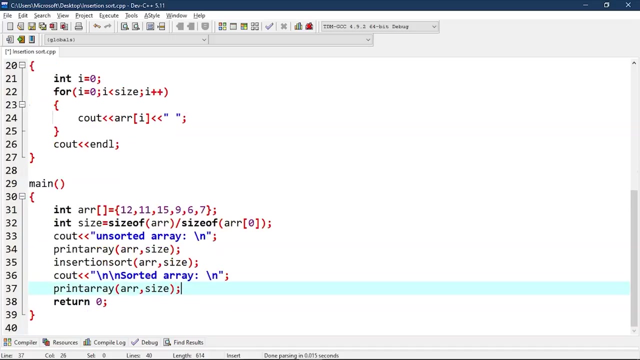 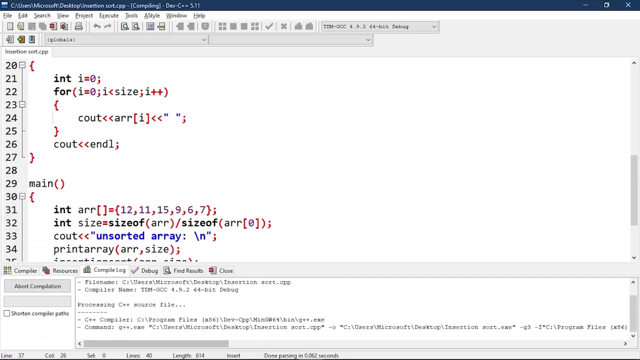 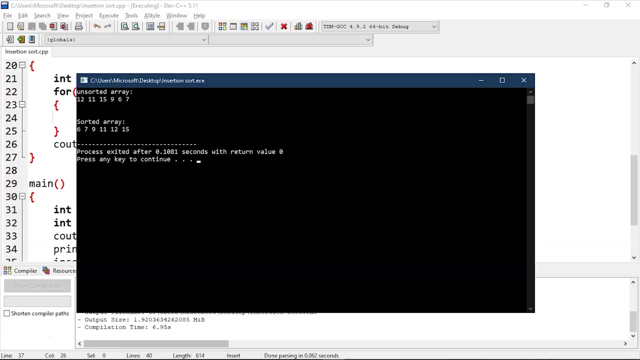 Now we will call insertion: sort: ARR comma size. see out, we will print this array sorted. now we will again call print array argument as ARR comma size. now let's print this. as you can see, our function is working flawlessly. it has sorted this array. let's get back to our slides. 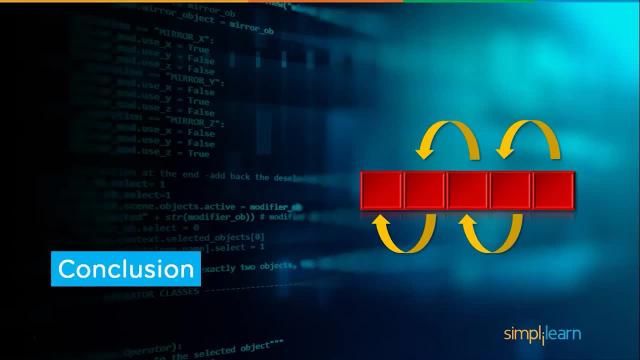 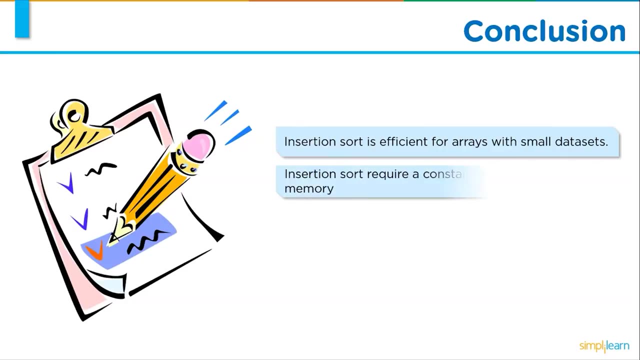 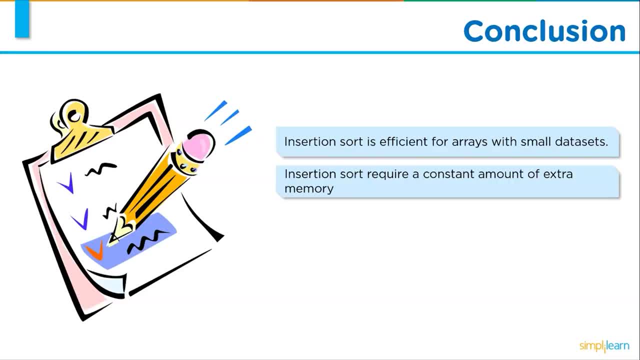